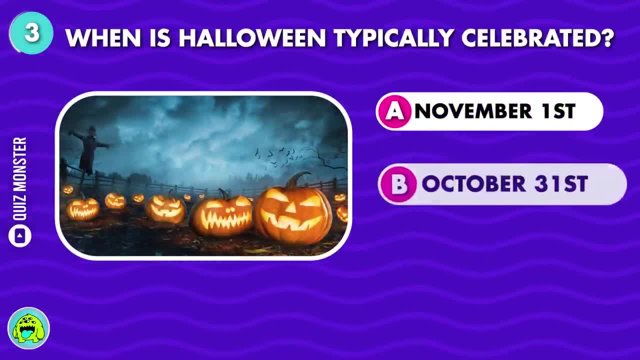 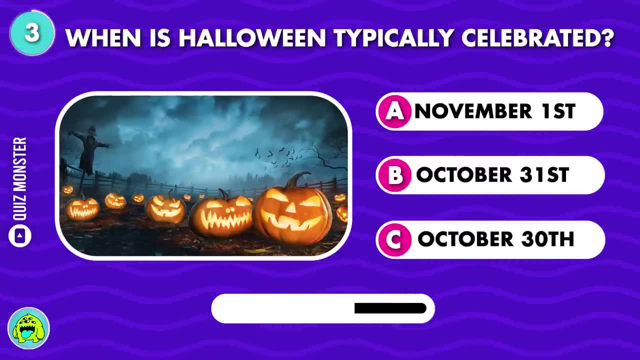 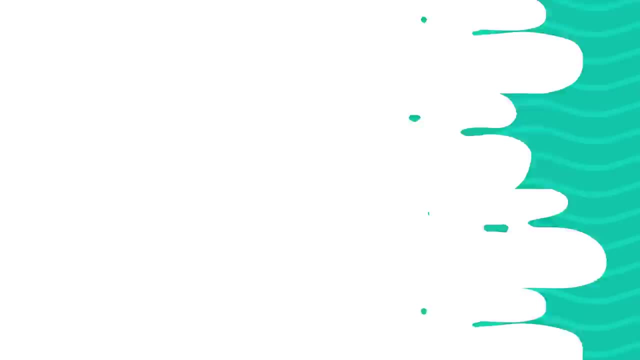 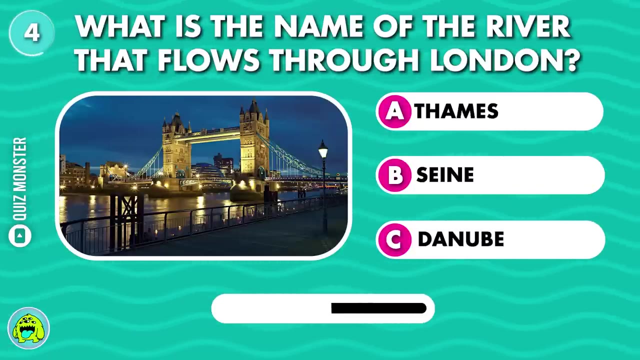 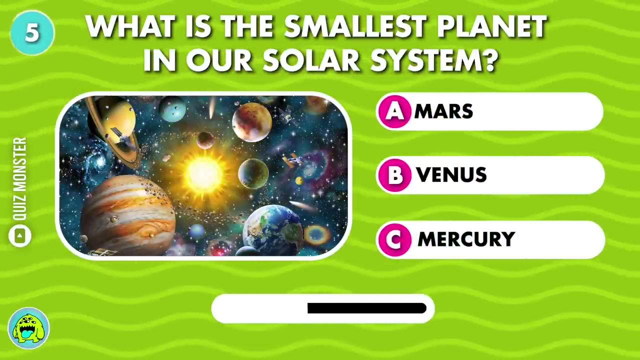 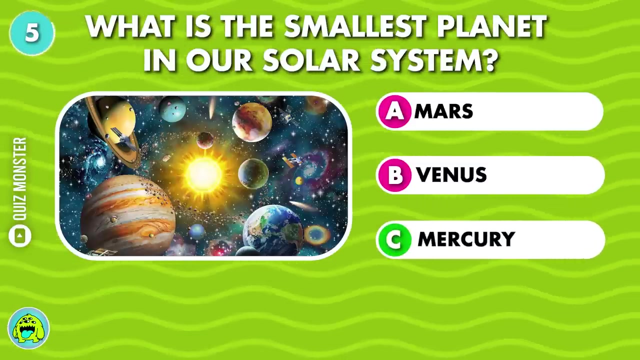 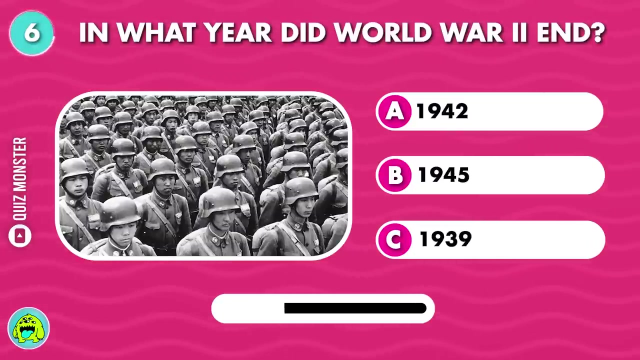 Photosynthesis. When is Halloween typically celebrated? October 31st. What is the name of the river that flows through London? October 31st- Thames. What is the smallest planet in our solar system- Mercury. In what year did World War II end? 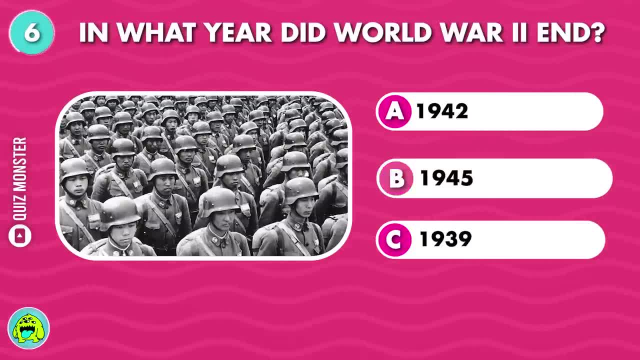 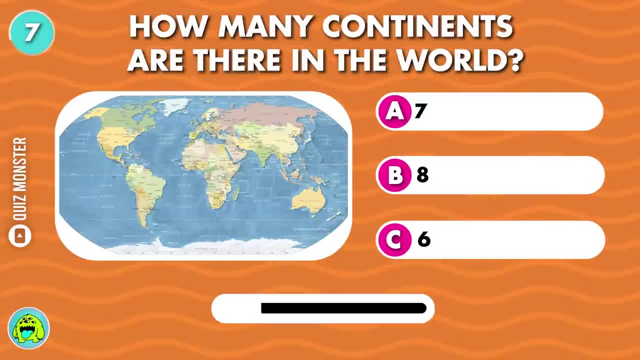 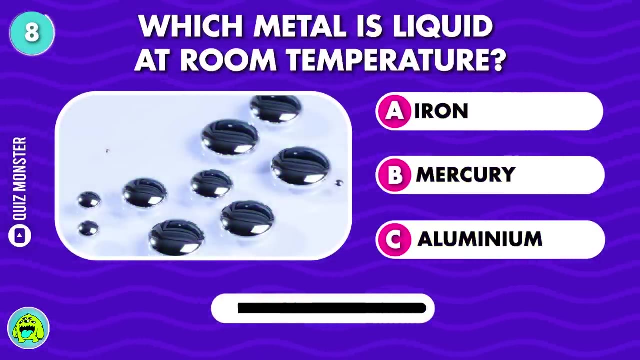 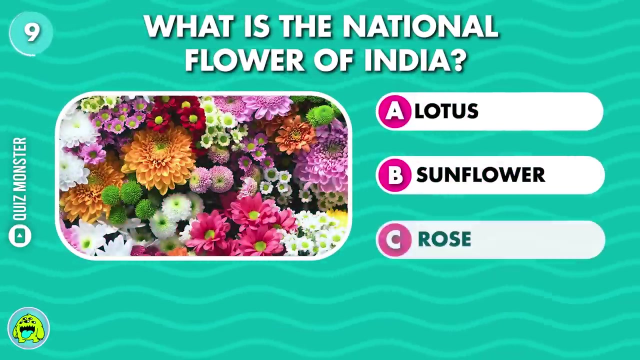 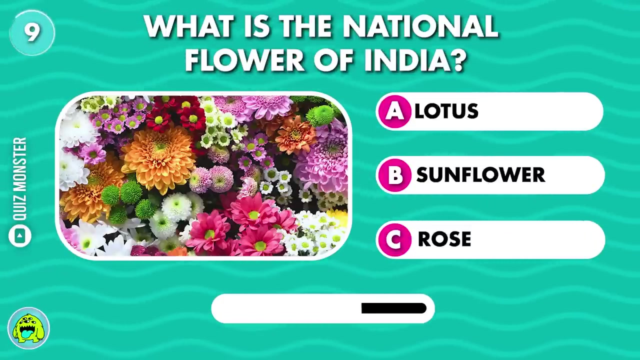 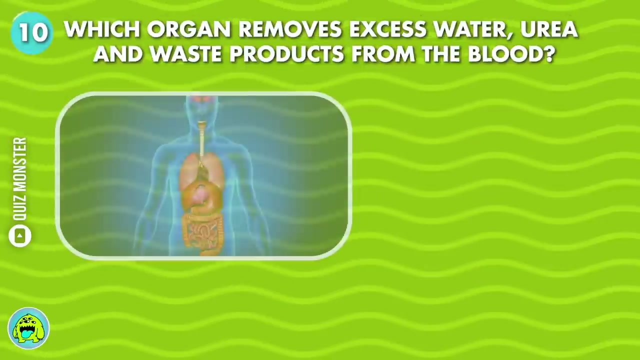 1945!, 1945!. How many continents are there in the world? Seven. Which metal is liquid at room temperature? Mercury, Mercury. What is the national flower of India? Lotus? Which organ removes excess water, urea and waste products from the blood? 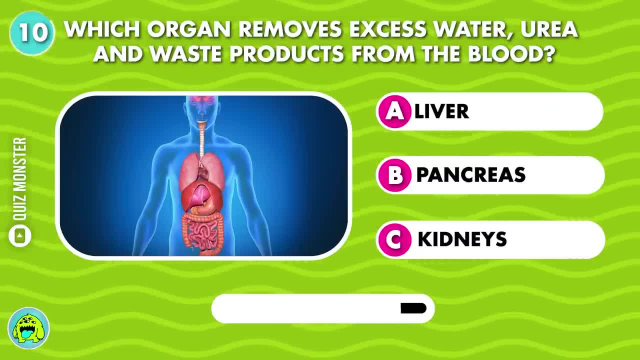 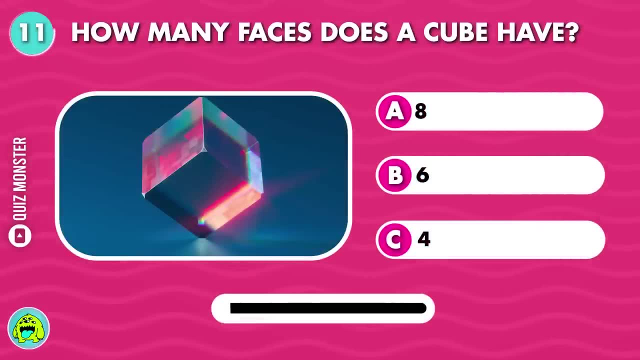 Lotus, Which organ removes excess water, urea and waste products from the blood. Lotus, Kidneys, The departing water, in which the water is taken off fuego. How many faces does a cube have? Six Heart Heart. 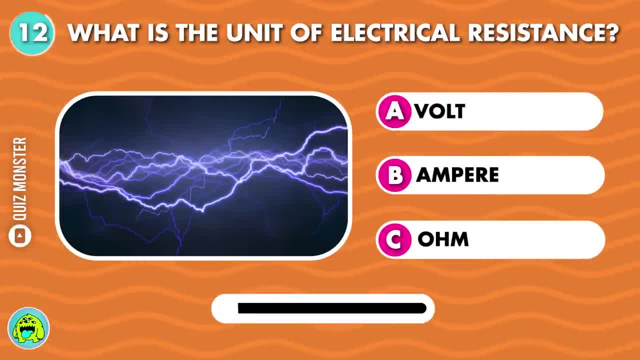 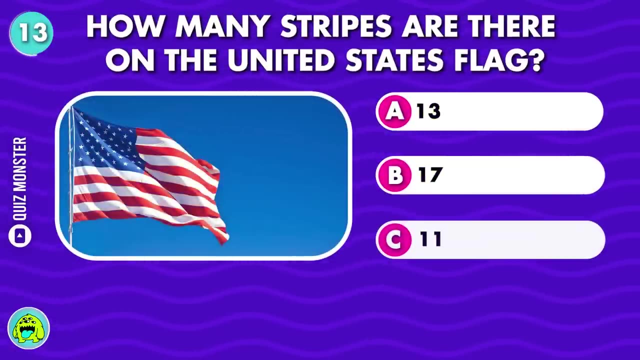 I don't want to know it. yet Why do we have six faces? What is the unit of electrical resistance Power, The numberすご? For what reason does a liquid make up the projecting气? Ohm? How many stripes are there on the United States flag? 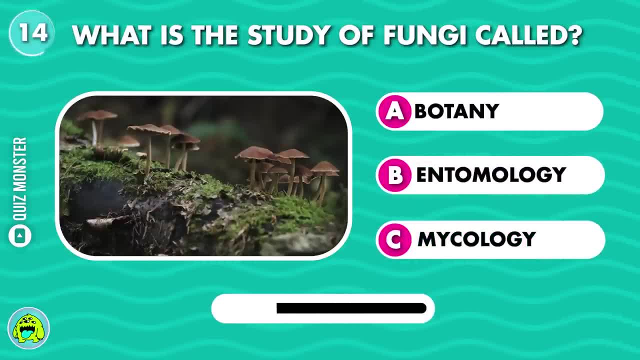 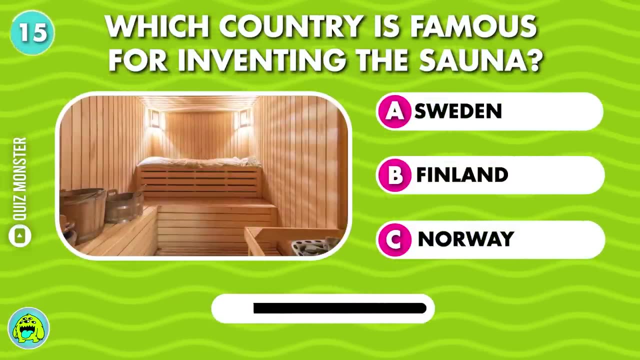 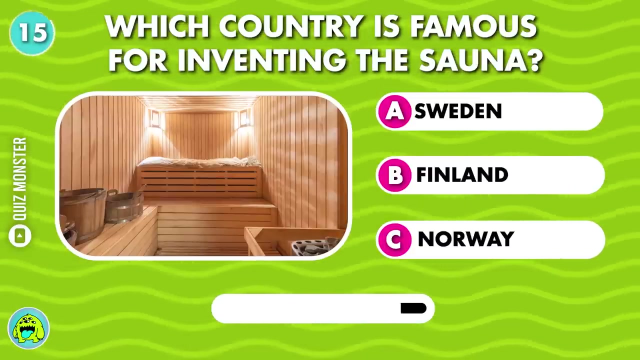 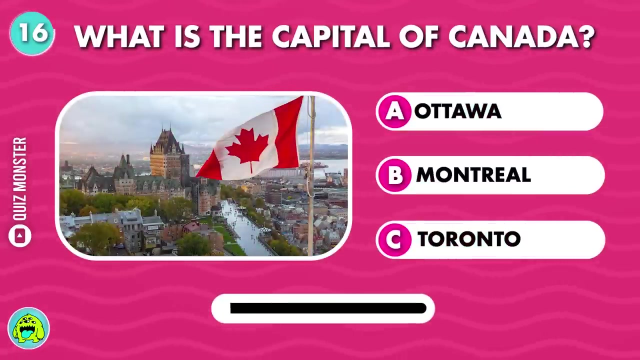 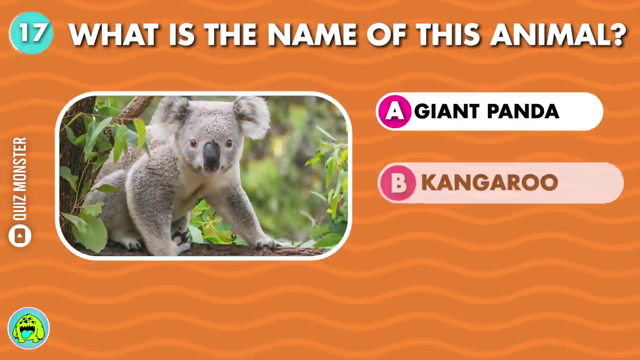 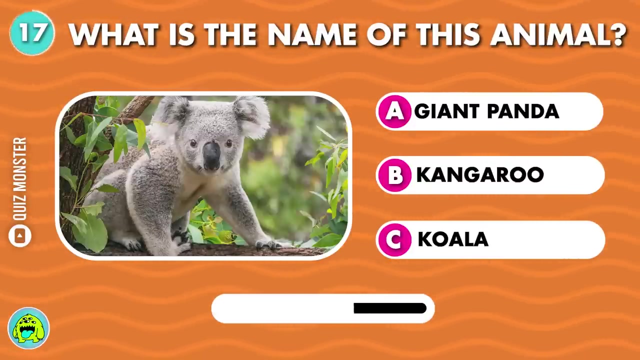 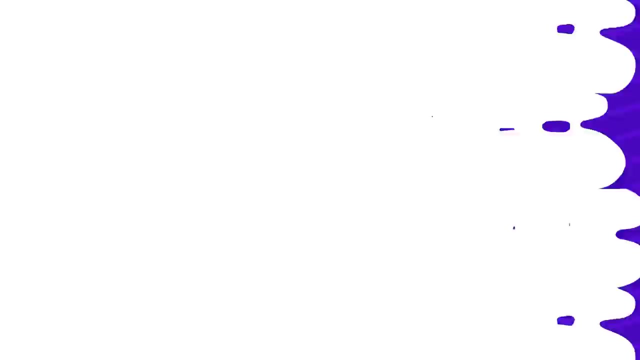 Thirteen, What is the study of fungi called Micology? Which country is famous for inventing the sauna, Finland. What is the capital of Canada, Ottawa. What is the name of this animal? Koala From the sun? which plant is the best? 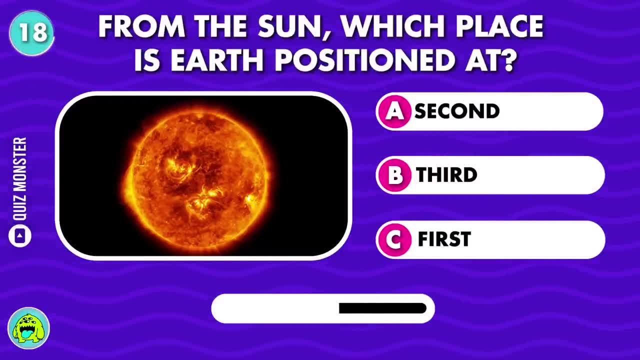 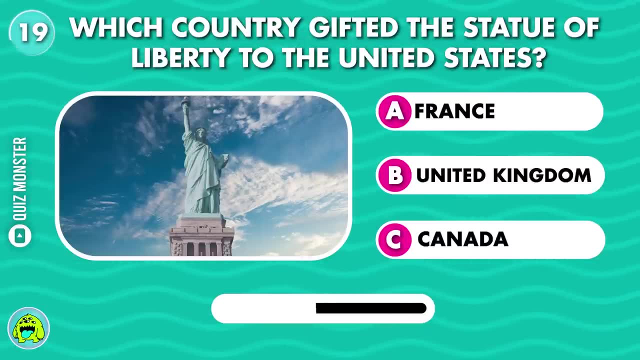 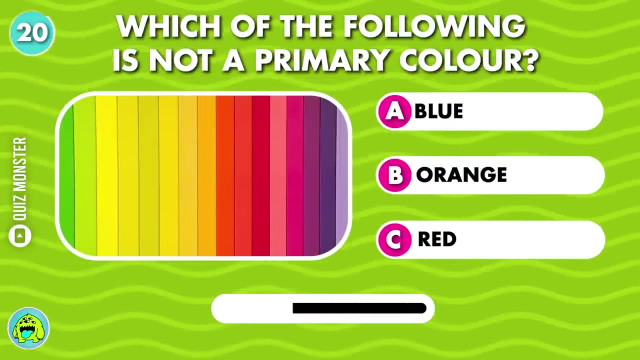 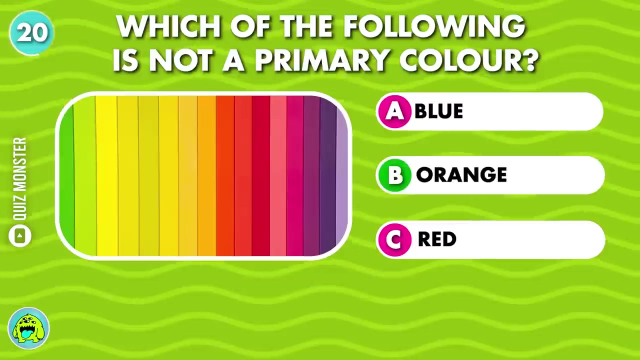 Earth? Which planet is Earth positioned at? Third, Which country gifted the Statue of Liberty to the United States? France, France. Which of the following is non-existent, France, What is its primary colour? Red, Red, Green, Green, Yellow, Green, Black, Blue, Blue, Red, Red, Blue, Blue. 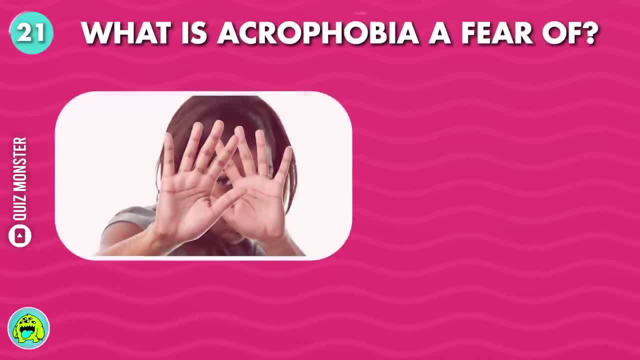 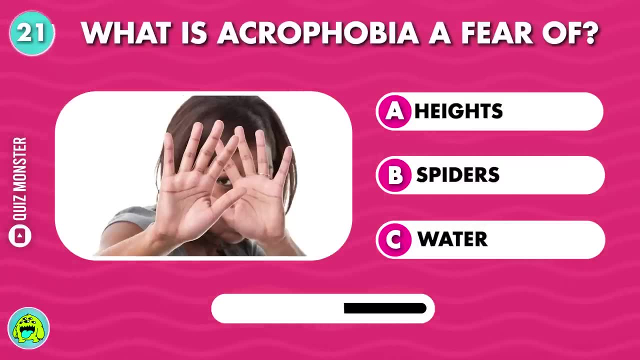 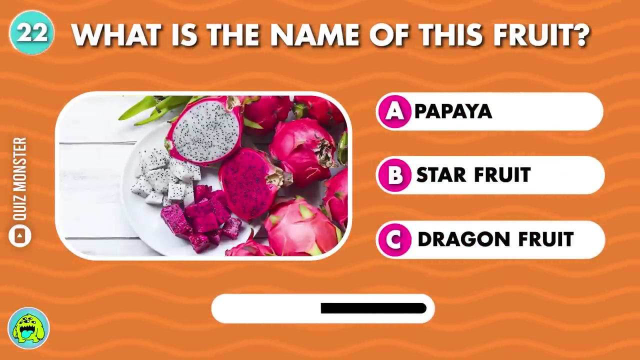 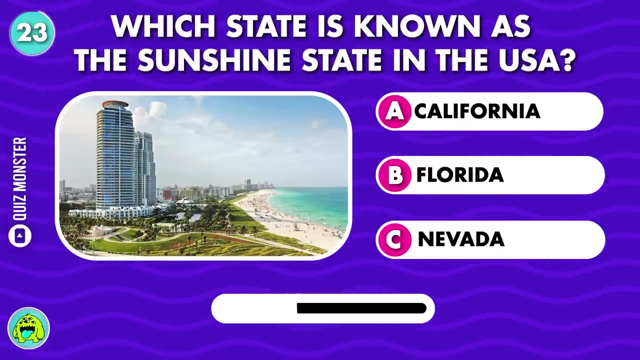 Blue, Pink, Blue, Blue, Green, Green, Blue, Green, Blue, Red, Blue, Green, Yellow, Pink, Blue, Yellow, Brown, Brown, Yellow, White, Pink, Blue, Black, Purple, Green, Blue, White, Grey, White, White, Orange, Orange, Yellow, Orange, Blue, Black, Blue. What is acrophobia of fear of Heights fruit, Dragon fruit? Which state is known as the sunshine state in the USA, Florida? 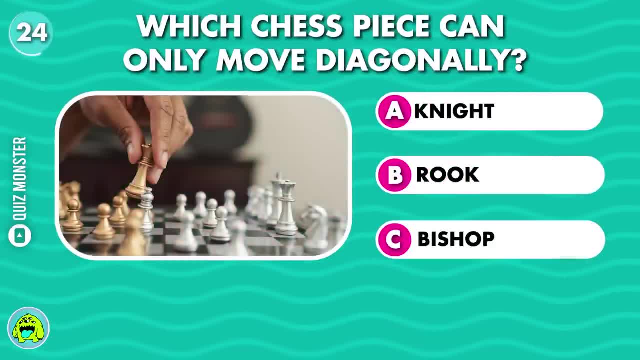 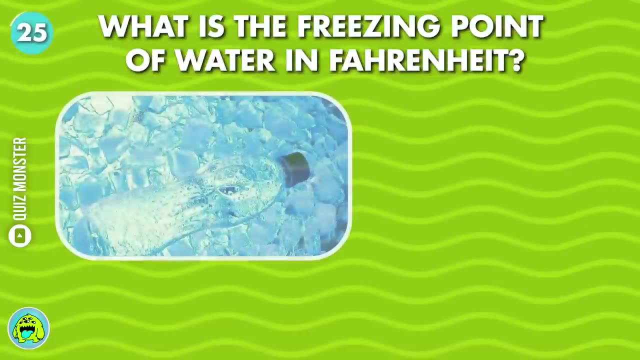 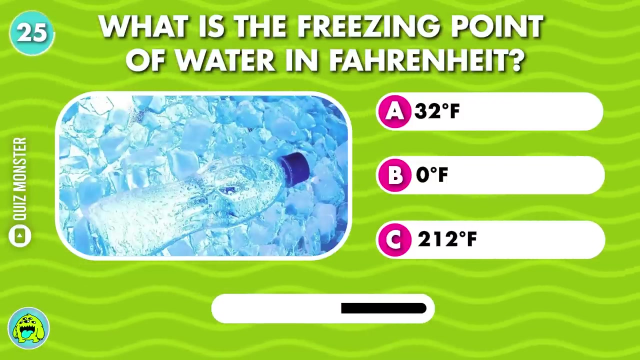 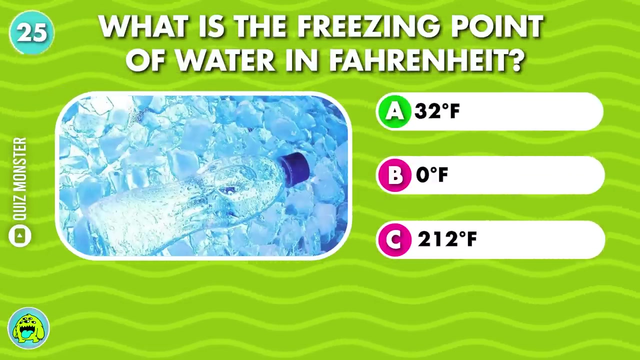 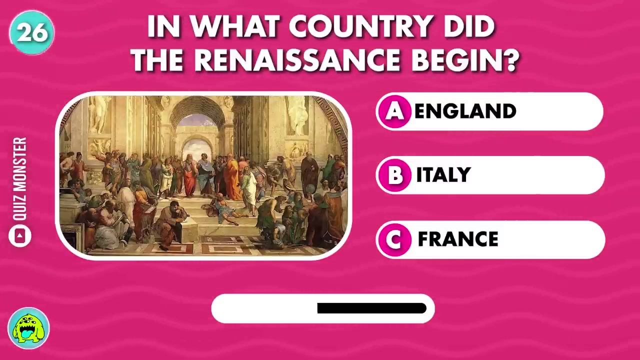 Which chess piece can only move diagonally. Bishop, What is the freezing point of water in Fahrenheit? Naturally, 32 degrees Fahrenheit. In what country did the Renaissance begin? Italy. What is the name of the mountain range in Celsius Manifesto? 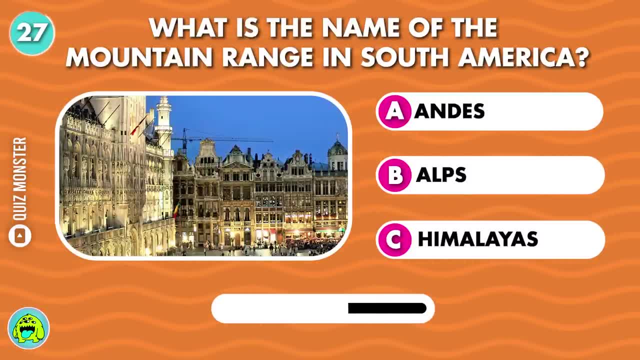 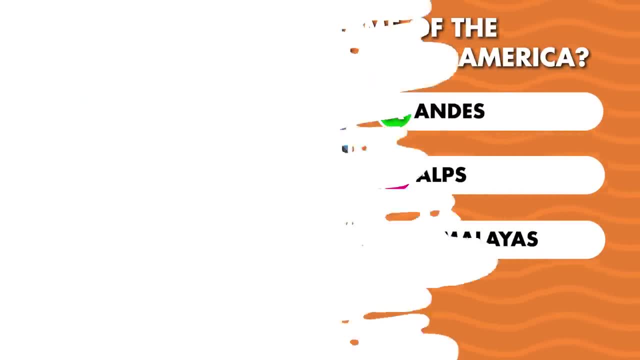 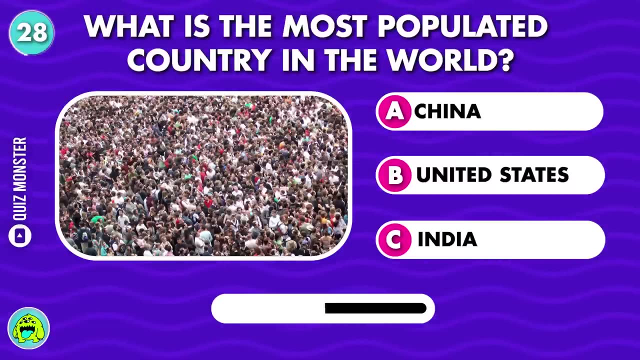 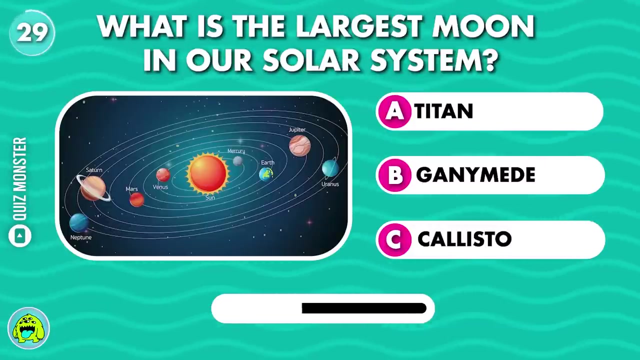 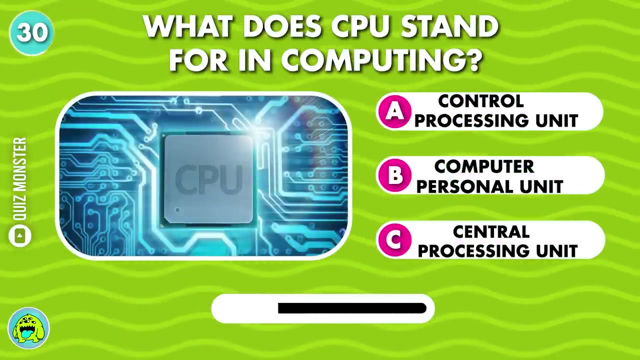 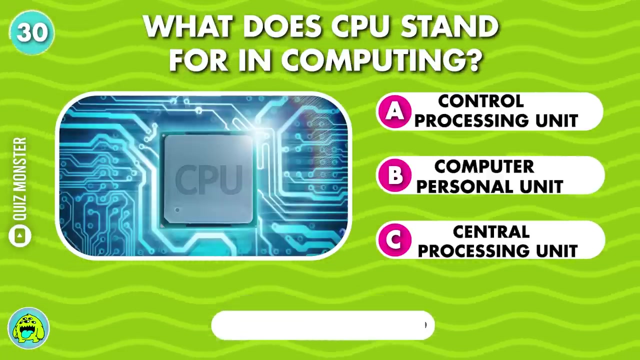 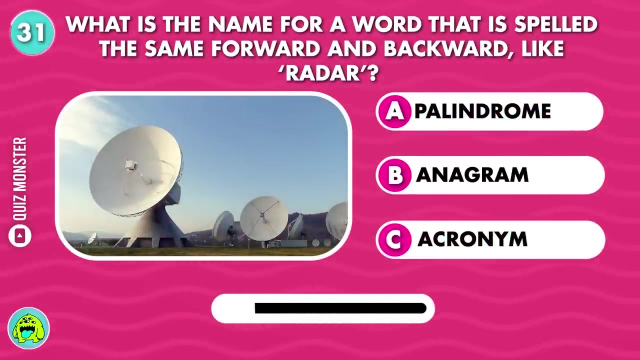 South America- Andes. What is the most populated country in the world- India. What is the largest moon in our solar system, Canomede. What does CPU stand for in computing? Central Processing Unit? What is the name for a word That is spelled the same forward and backward, like radar? Palindrome. In which city is the Colosseum located? Rome? Who is this athlete? The Colosseum is located at the center of the Earth's atmosphere. The Colosseum is located at the center of the Earth's atmosphere. 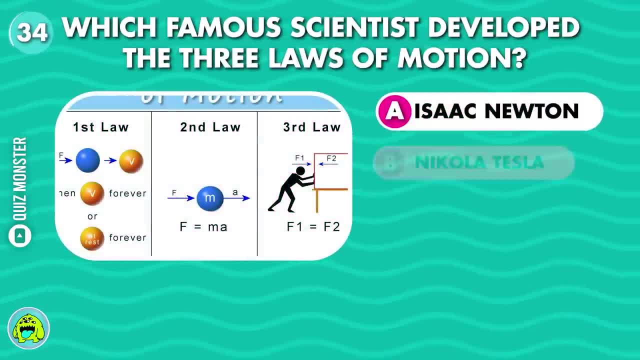 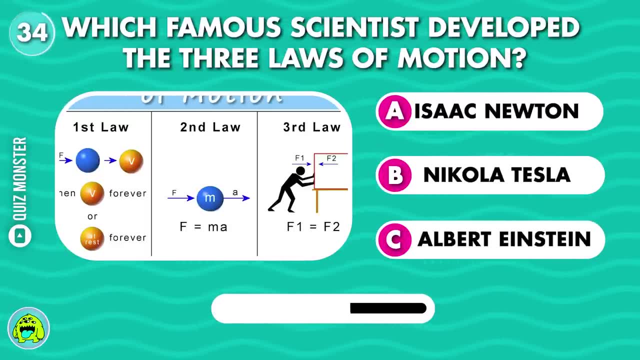 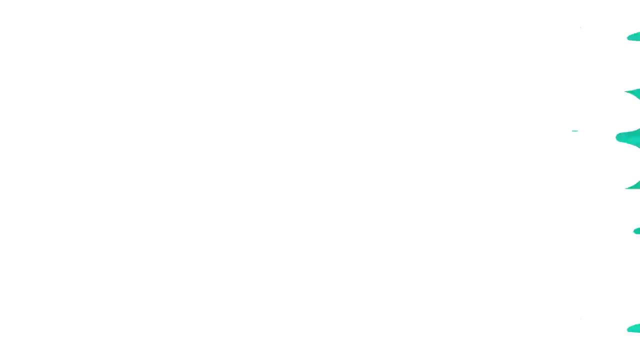 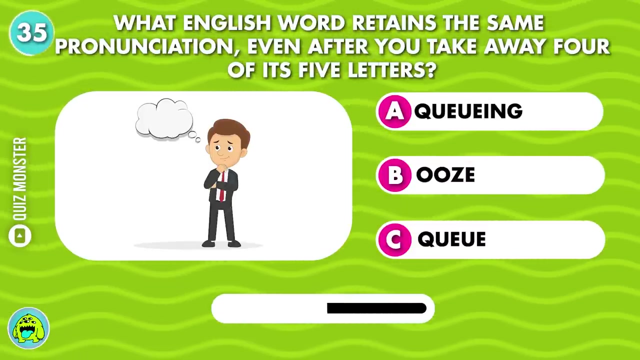 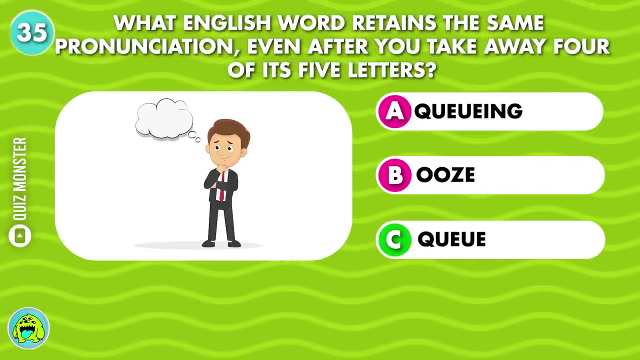 The Colosseum is located at the center of the Earth's atmosphere. Michael Jordan: Which famous scientist developed the three laws of motion? Isaac Newton: What English word is the most common word? in English word Q. What is the name of this currency? 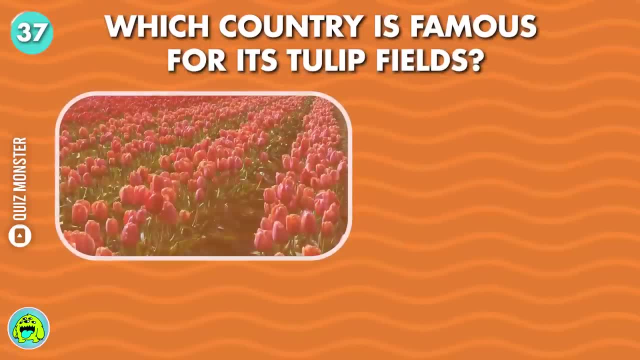 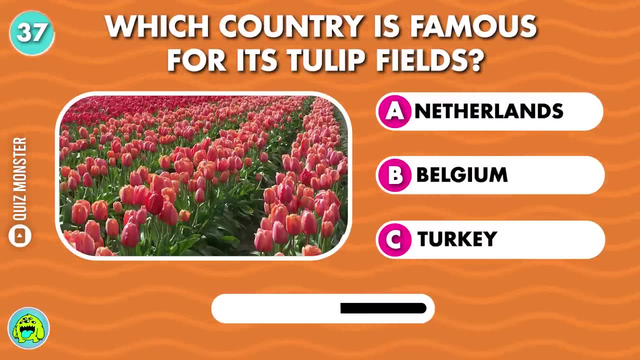 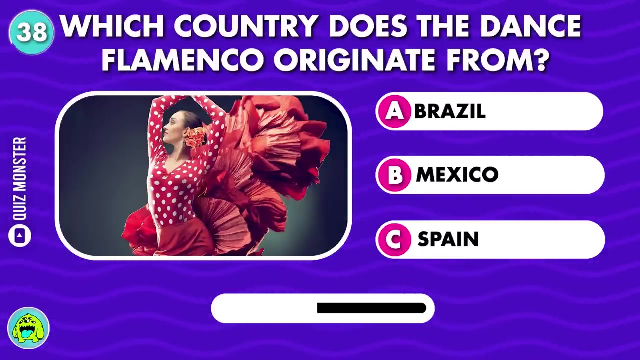 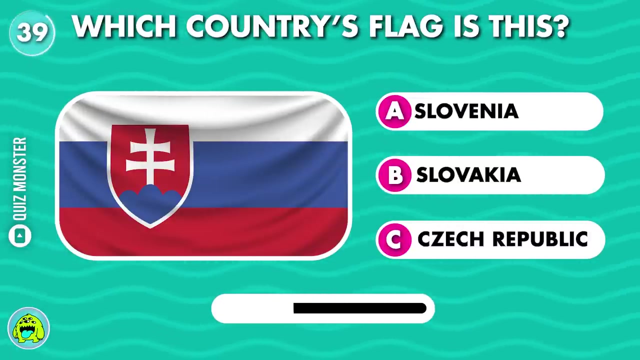 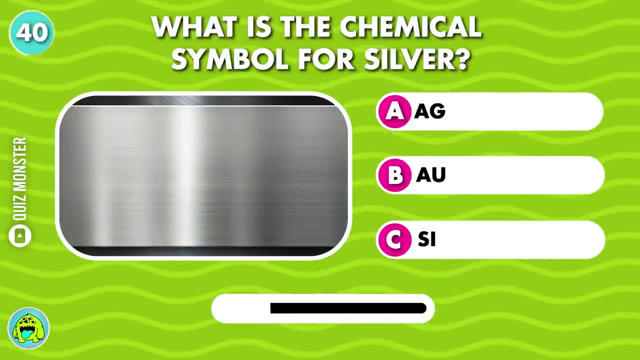 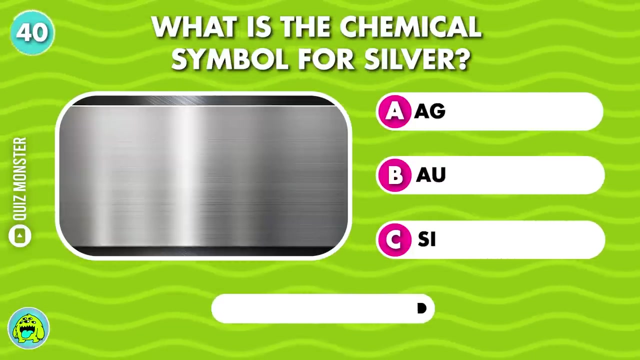 Euro. Which country is famous for its tulip fields? Netherlands. Which country does the dance flamenco originate from? Spain? Which country does the dance flamenco originate from? Which country's flag is this: Slovakia? What is the chemical symbol for silver AG? 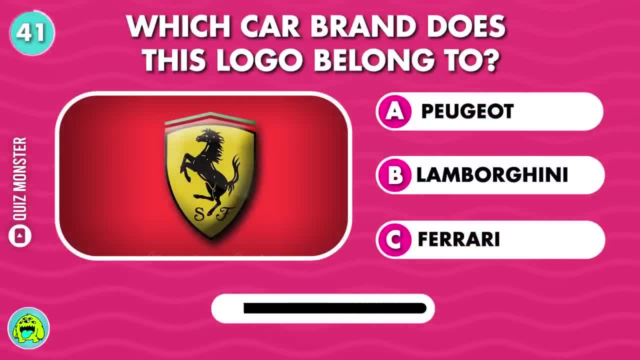 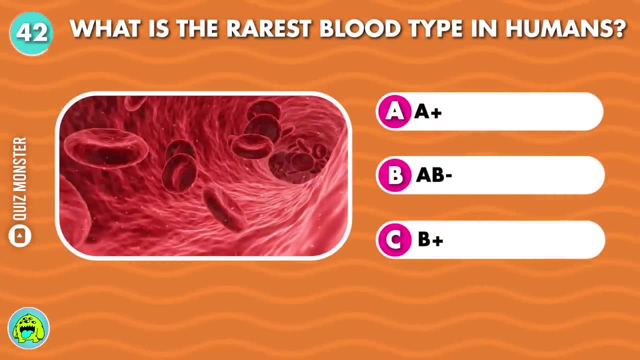 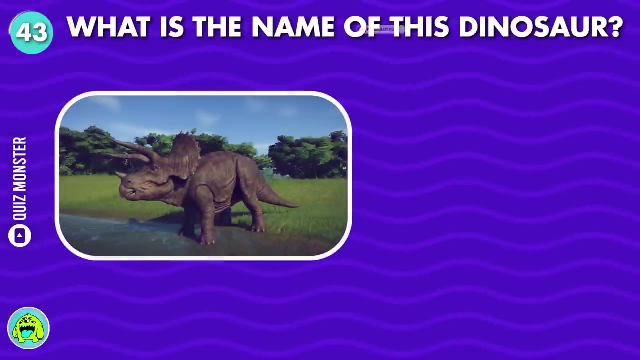 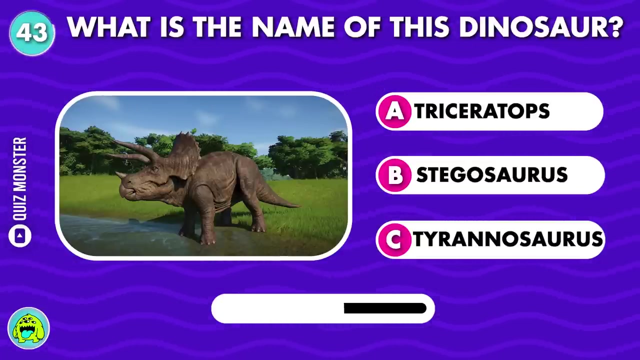 Which car brand does this logo belong to? Ferrari? What is the rarest blood type in humans? A, B Minus. What is the name of this dinosaur, Triceratops? Which planet has the most moons in the world? Italy? Which planet has the most moons in the world? 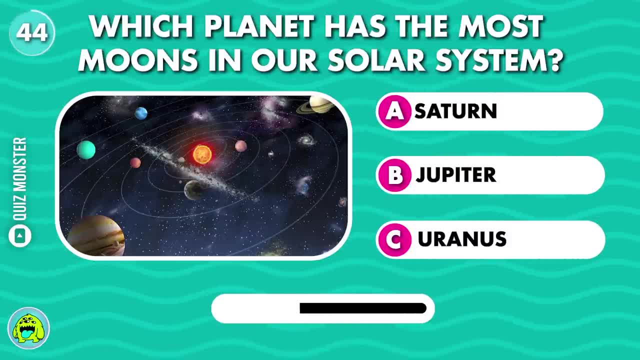 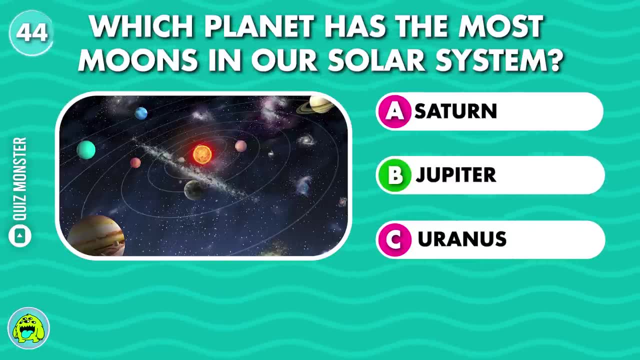 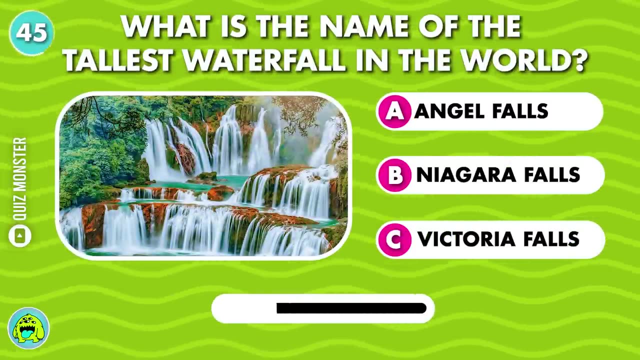 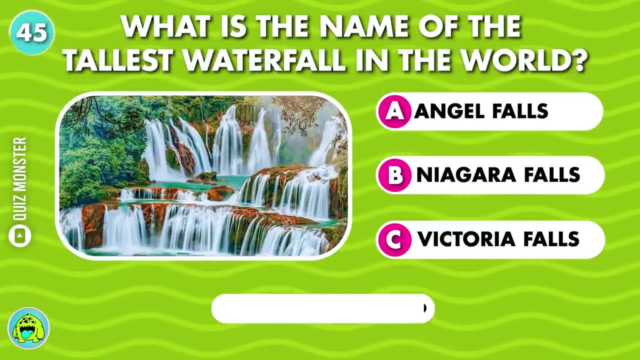 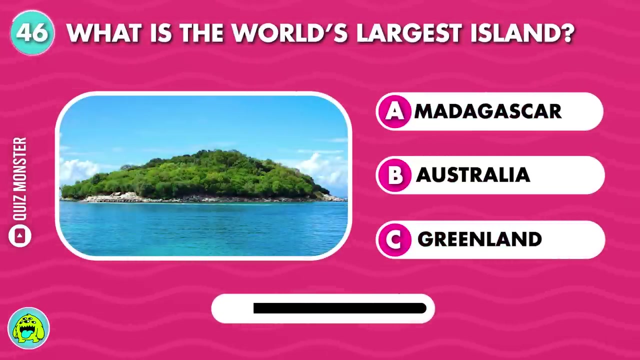 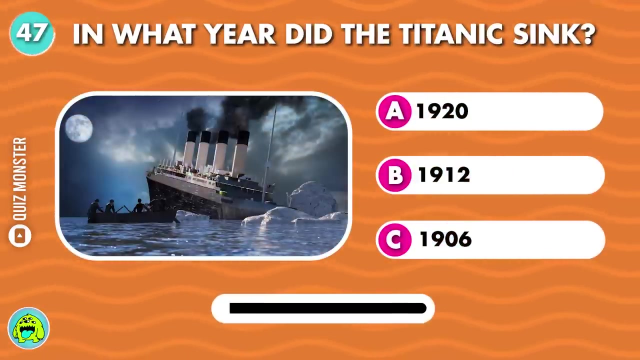 banyak. Which planet has the most moons in our solar system? Jupiter. What is the name of the tallest waterfall in the world? Angel Falls. What is the name of the tallest waterfall in the world? What is the world's largest island? Greenland. In what year did the Titanic sink? 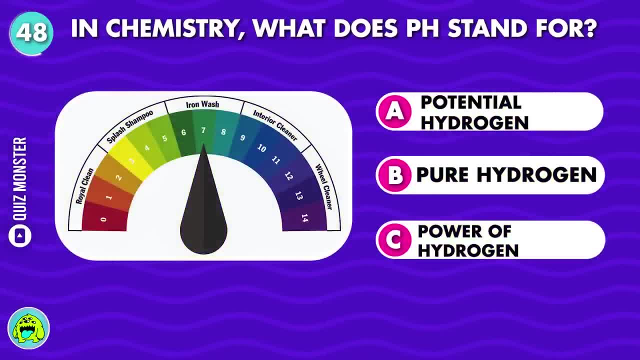 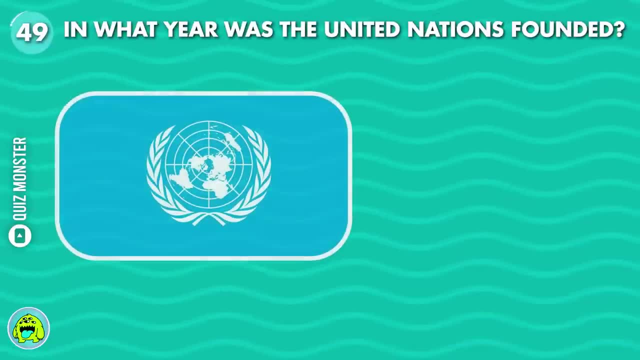 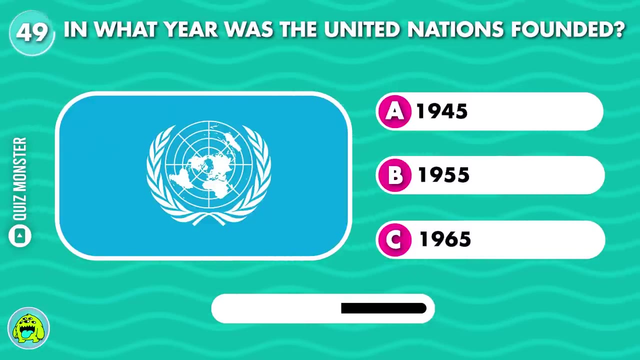 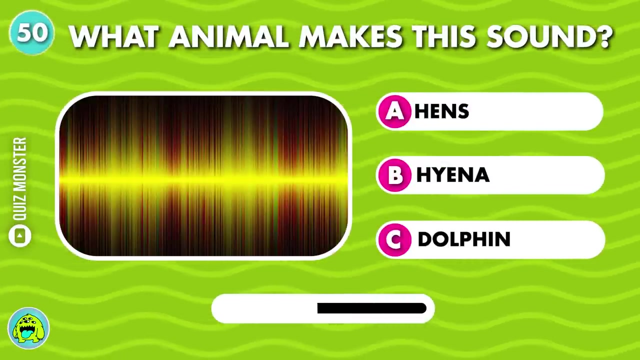 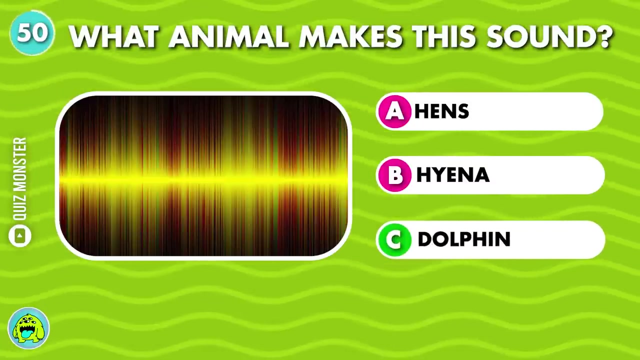 1912. In chemistry, what does pH stand for Power of hydrogen? In what year was the United Nations founded? 1945- 1945. In what year was the United Nations founded? 1912? What animal makes this sound Dolphin? What is the sum of angles in a triangle? 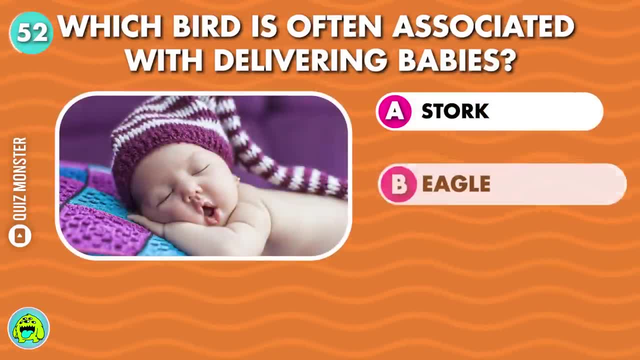 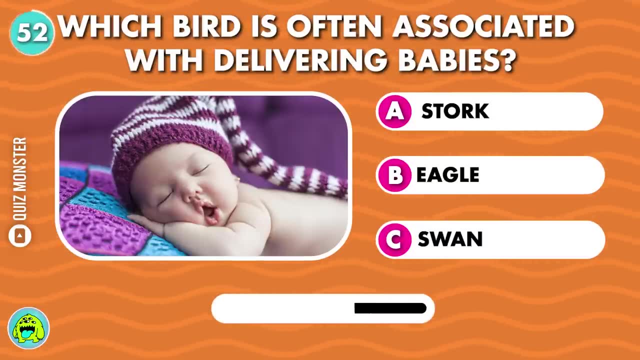 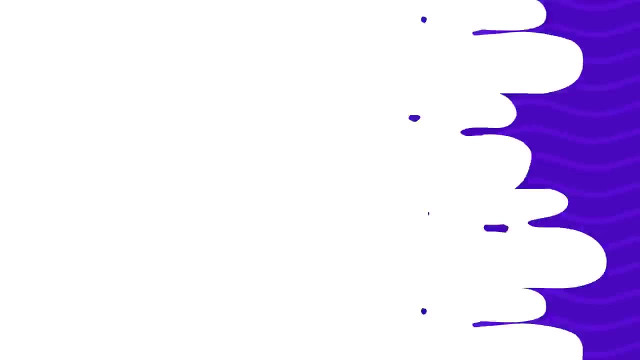 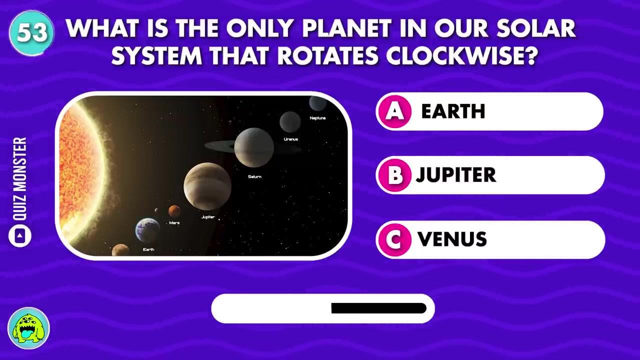 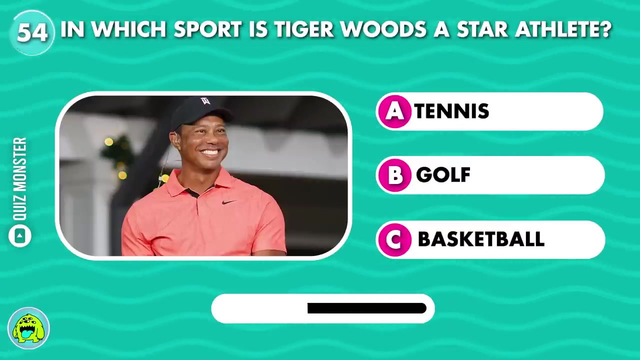 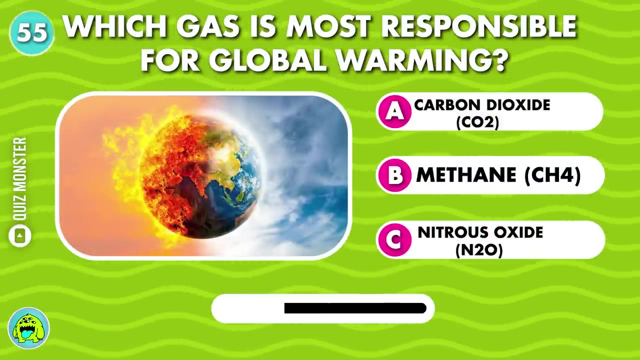 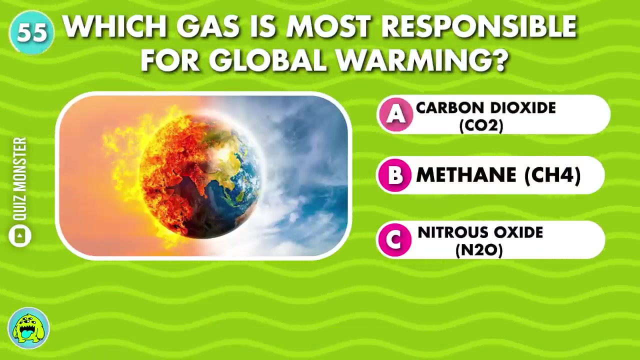 180 degrees. Which bird is often associated with delivering babies? Stork. What is the only planet in our solar system that rotates clockwise? Venus? In which sport is Tiger Woods a star athlete, Golf. Which gas is more responsible for global warming? Carbon dioxide or CO2? 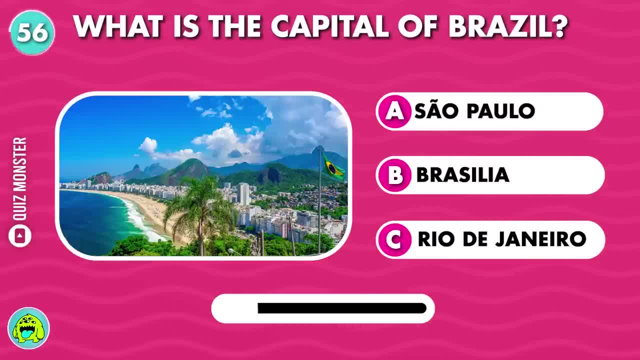 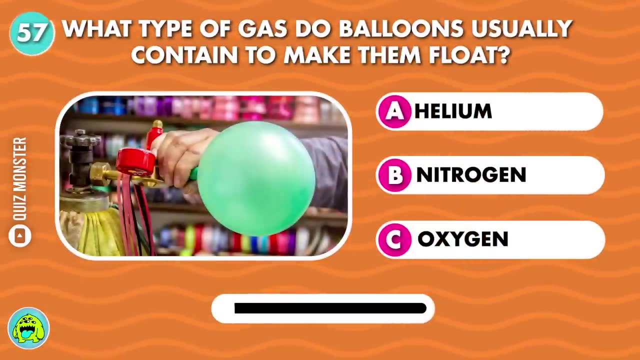 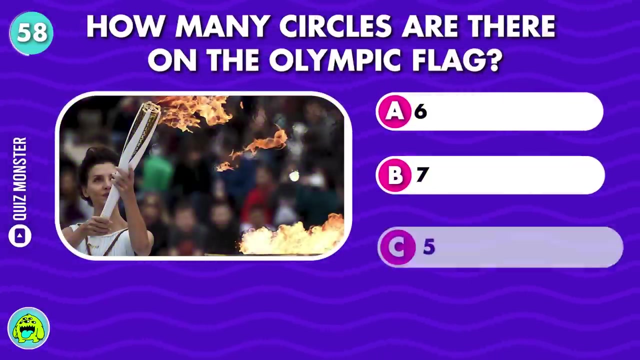 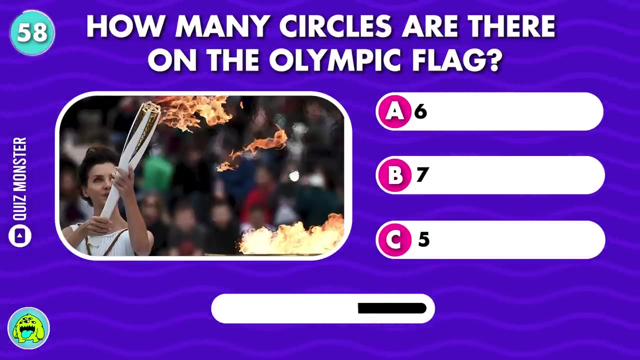 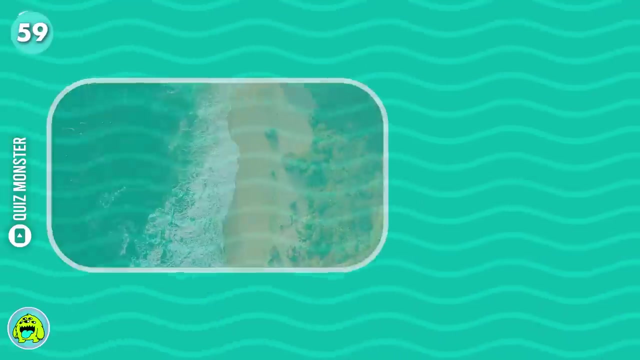 What is the capital of Brazil, Brazilia? What type of gas do balloons usually contain to make them Gas? Gas, Gas, Gas to make them float, Helium? How many circles are there on the Olympic flag Five? Which country has the longest coastline in the world? 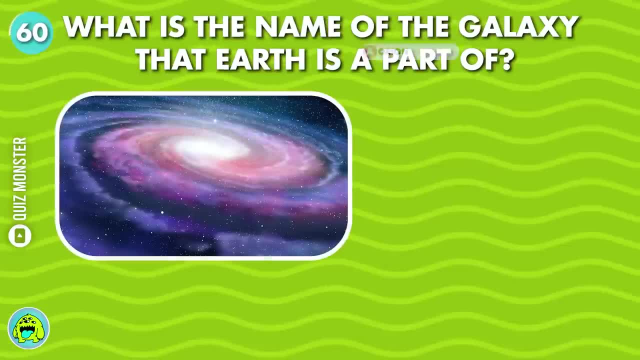 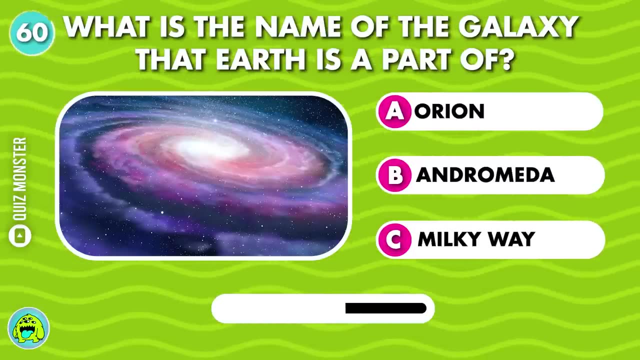 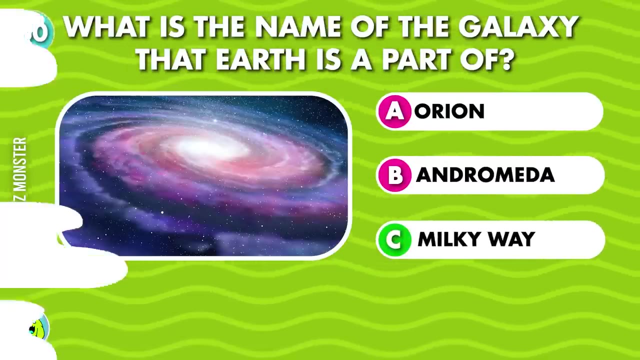 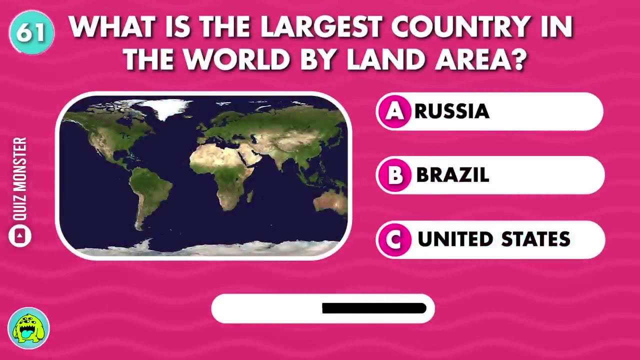 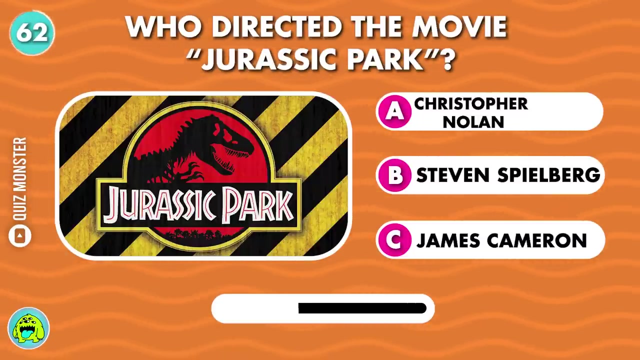 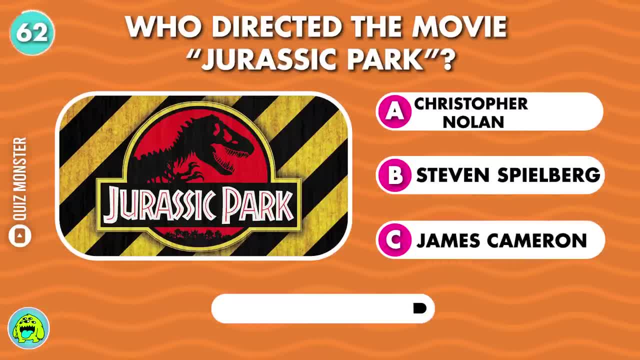 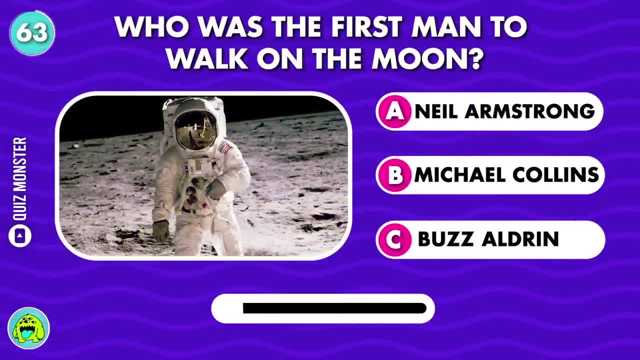 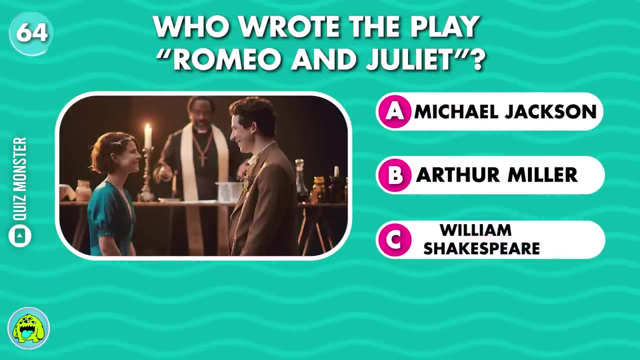 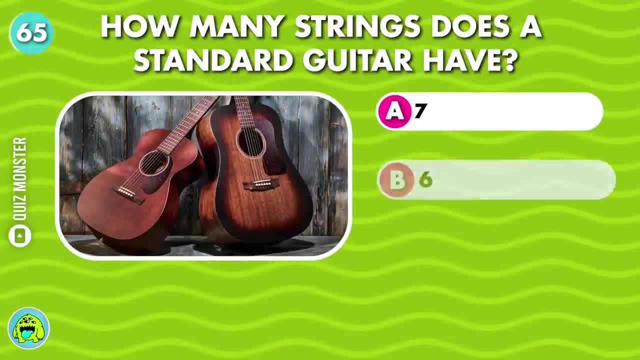 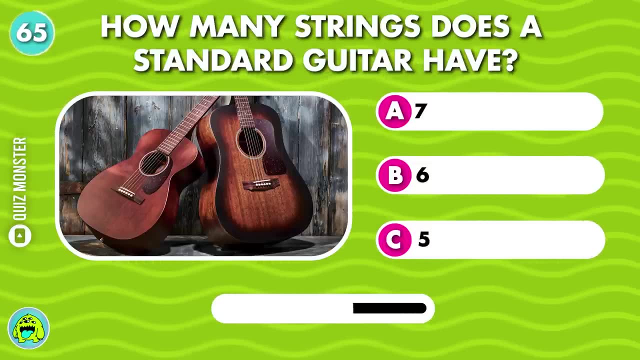 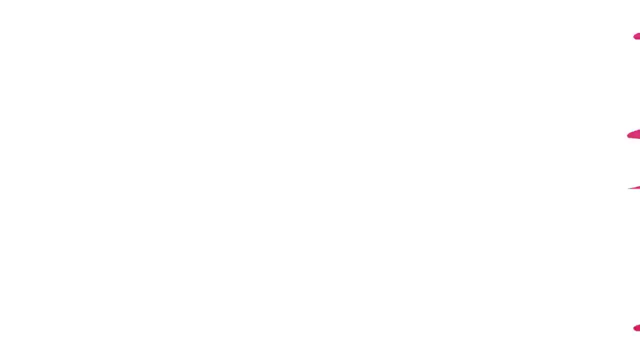 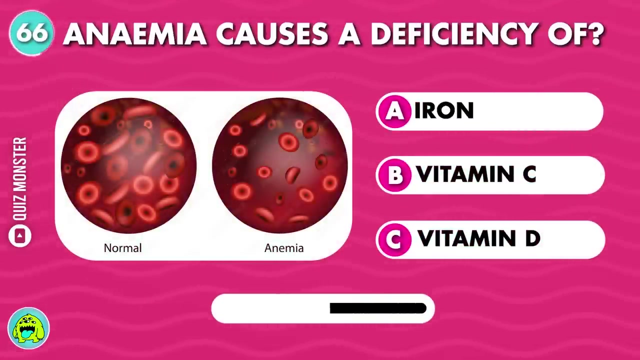 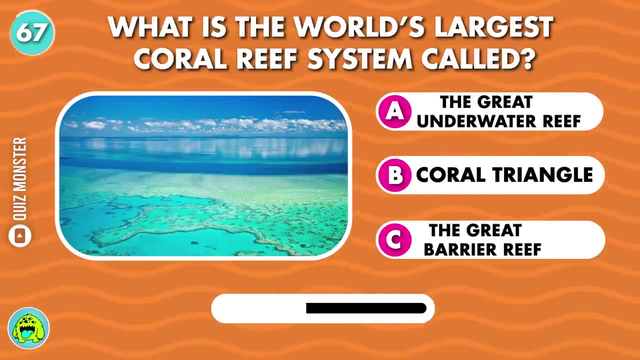 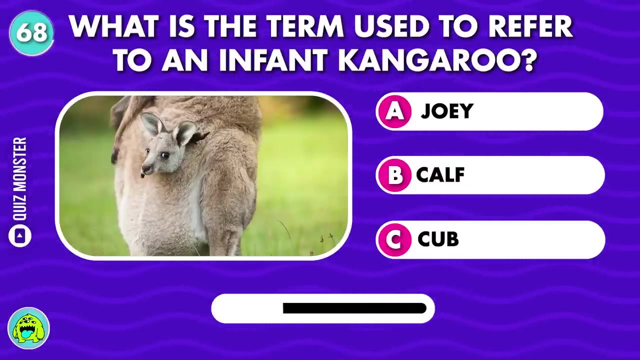 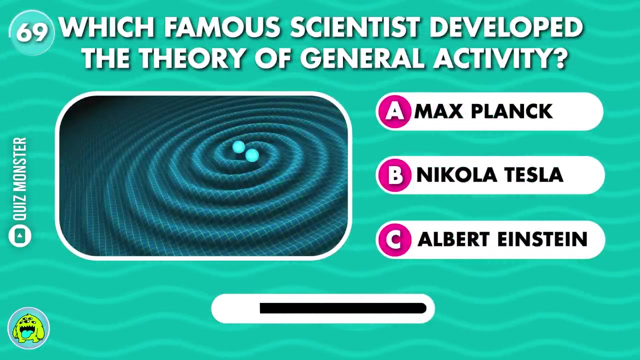 William Shakespeare. How many strings does a standard guitar have? Six Anemia causes a deficiency of Iron. What is the largest coral reef system, called The Great Barrier Reef? What is the term used to refer to an infant kangaroo, Joey? Which famous scientist developed the theory of general activity? 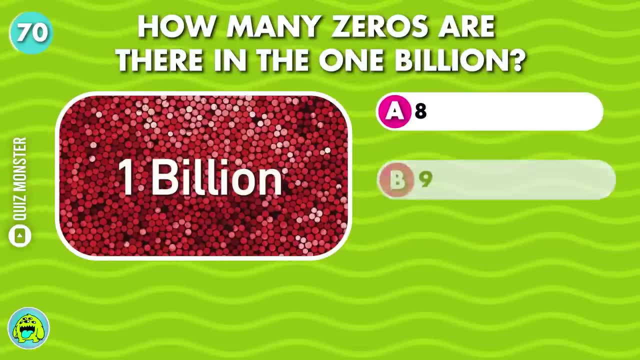 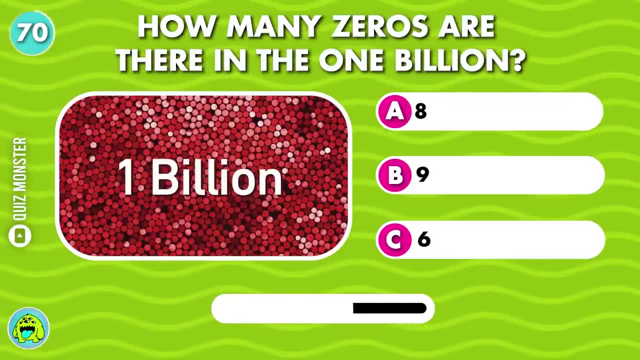 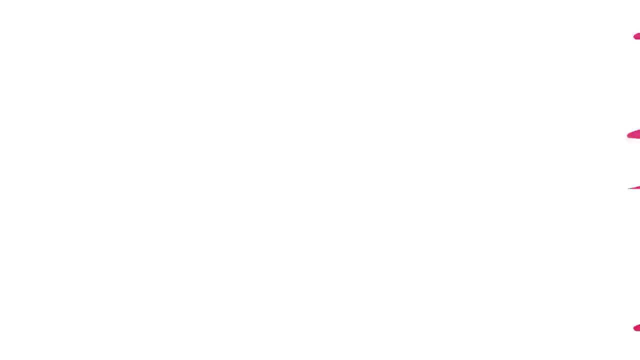 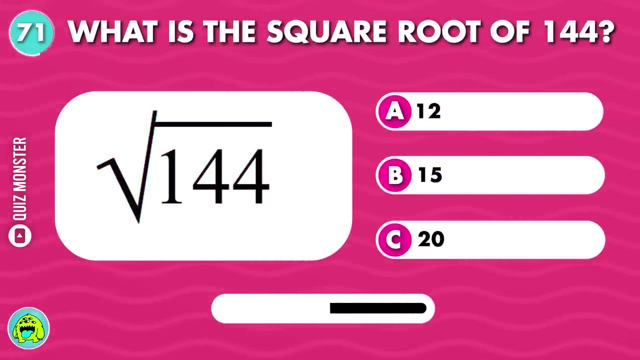 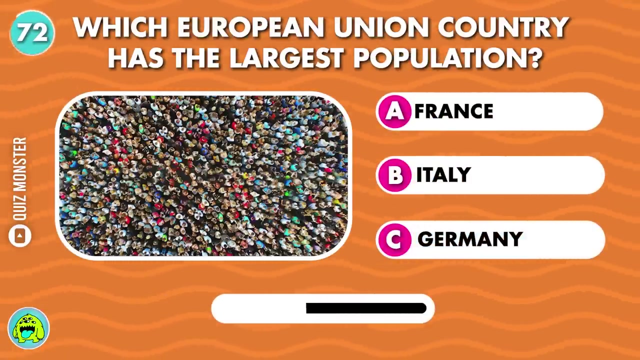 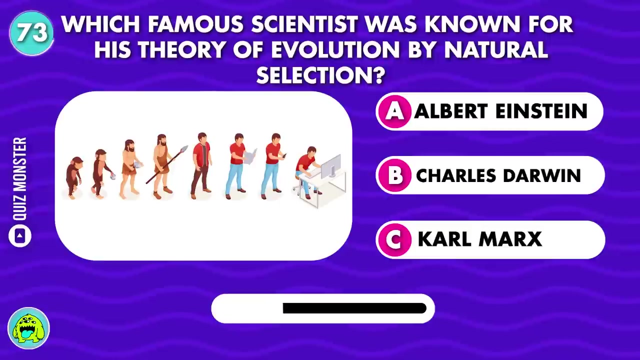 Albert Einstein. How many zeros are there in the one billion Nine? What is the square root of One hundred forty-four Twelve? Which European Union country has the largest population? Germany. What is the largest city in the world? Which famous scientist was known for his theory of evolution by natural selection? 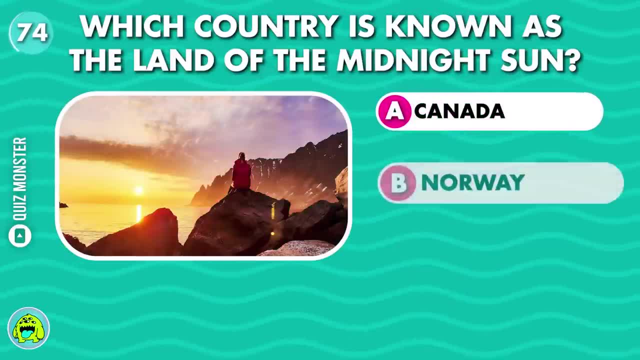 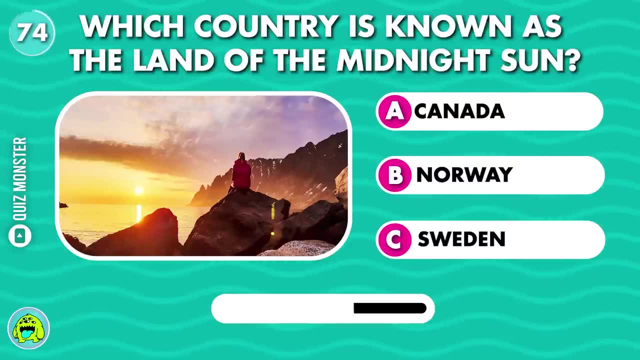 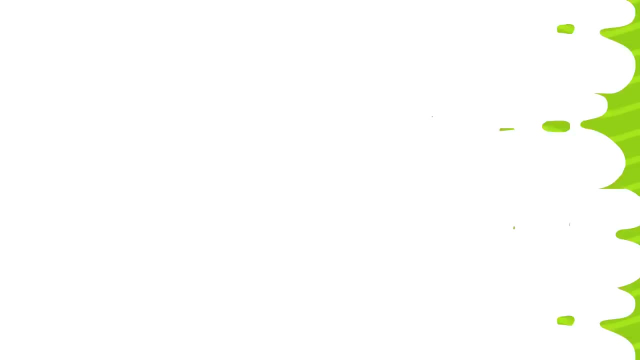 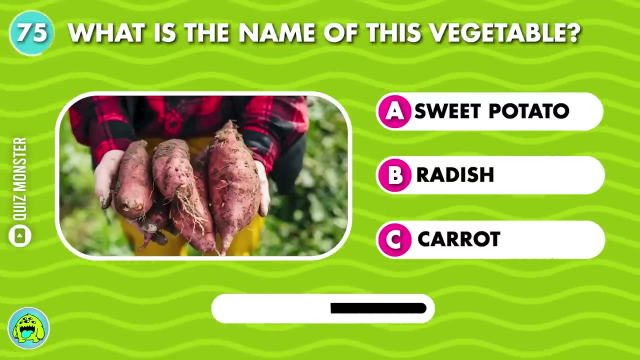 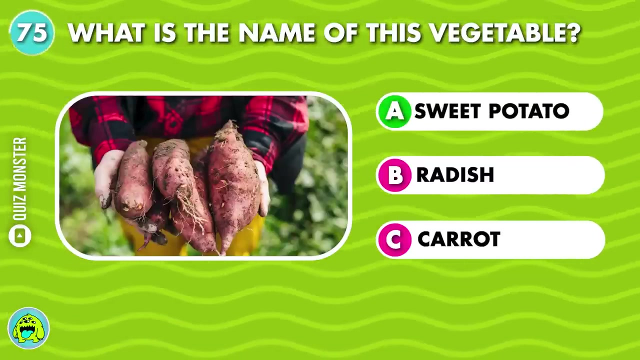 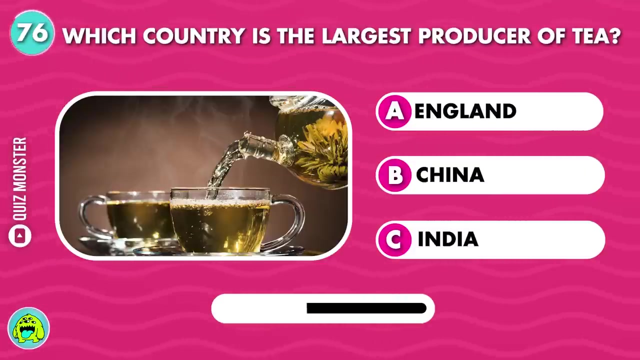 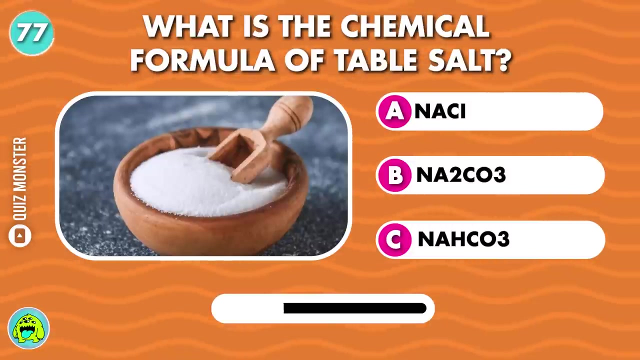 Charles Darwin. Which country is known as the Land of the Midnight Sun? Norway. What is the name of this vegetable? Sweet potato. Which country is the largest producer of tea? China. What is the chemical formula of table salt? N-A-C-L? What is this famous person? 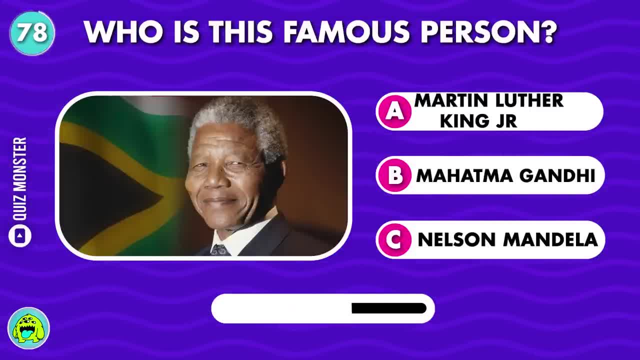 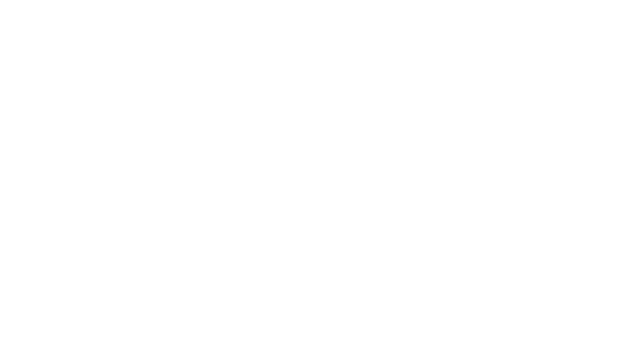 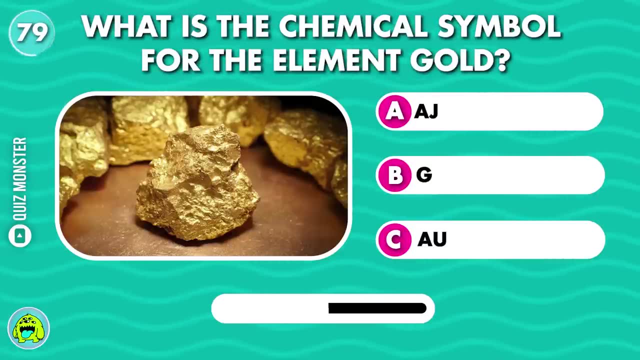 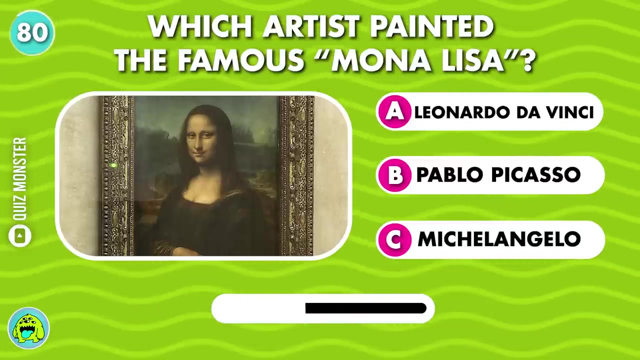 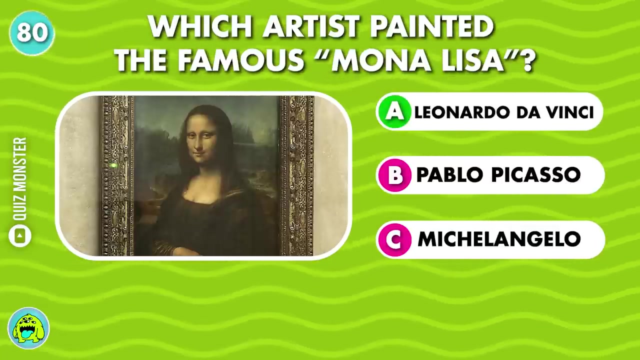 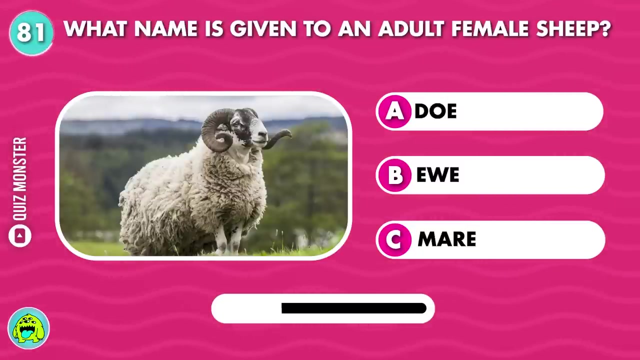 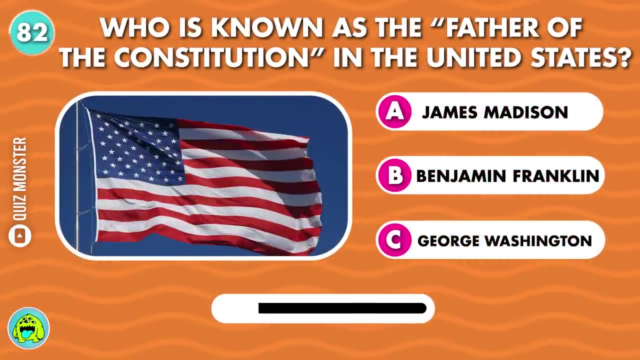 Nelson Mandela? What is the chemical symbol of the element gold? A-U? Which artist painted the famous painting, The famous Mona Lisa, Leonardo da Vinci? What name is given to an adult female sheep? U Who is known as the father of the cow Constitution in the United States? 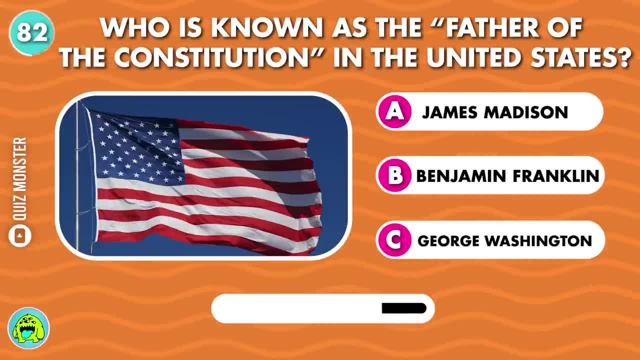 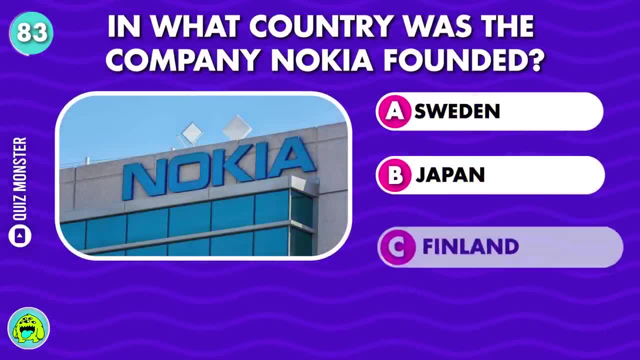 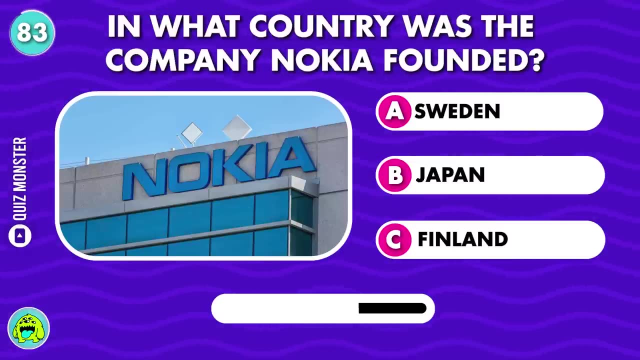 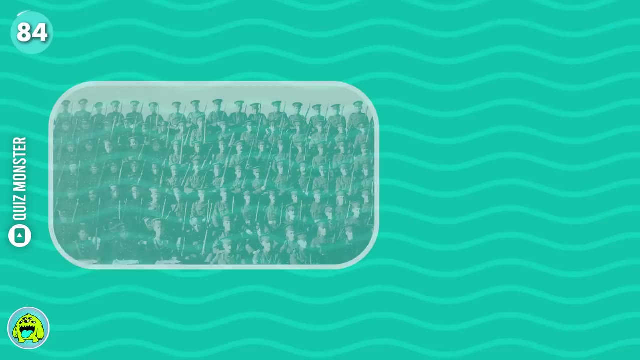 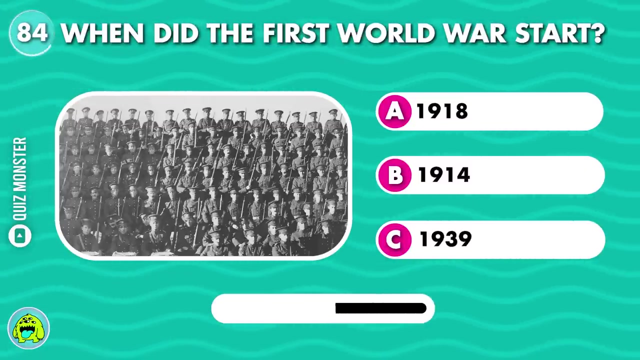 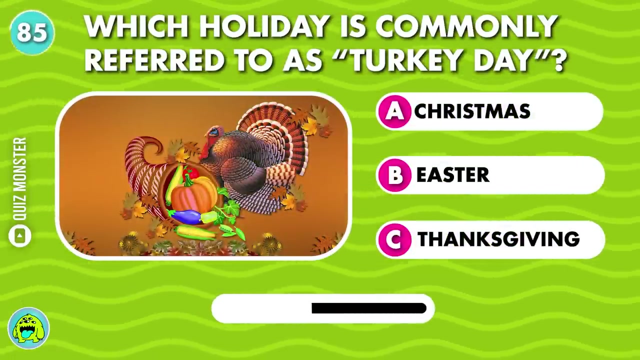 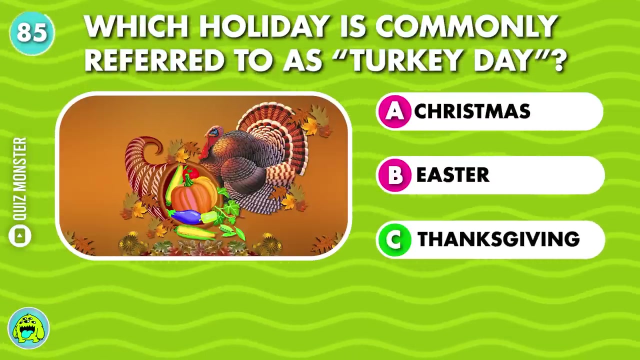 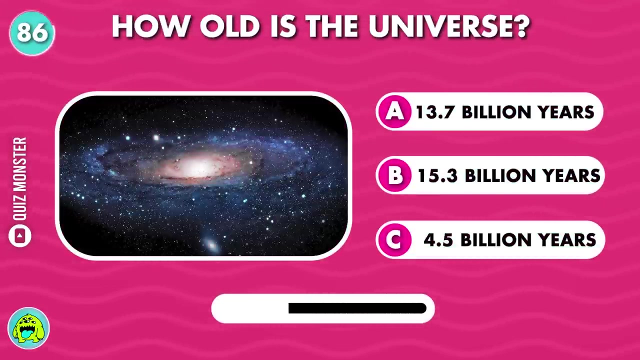 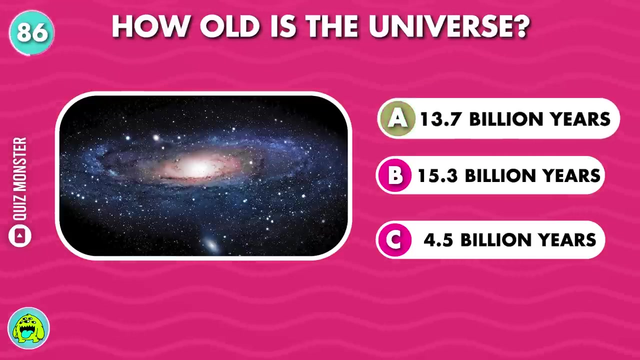 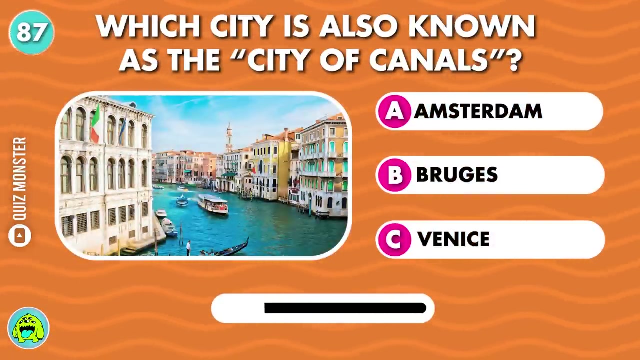 James Madison. In what country was the company Nokia founded? Finland? When did the First World War start? 1914? Which holiday is commonly referred to as Turkey Day, Thanksgiving, Thanksgiving? How old is the universe? 13.7 billion years. Which city is also known as the City of Canals? 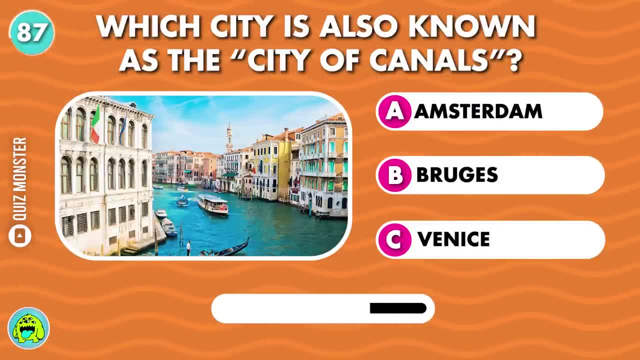 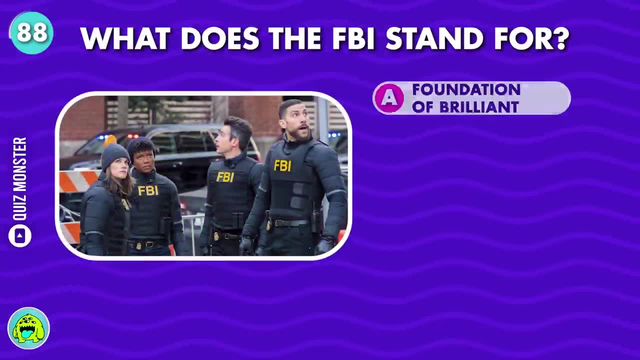 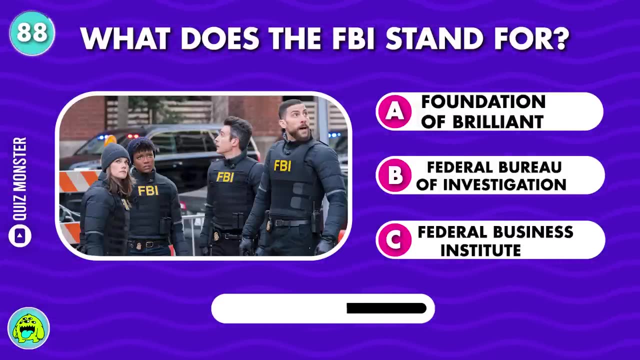 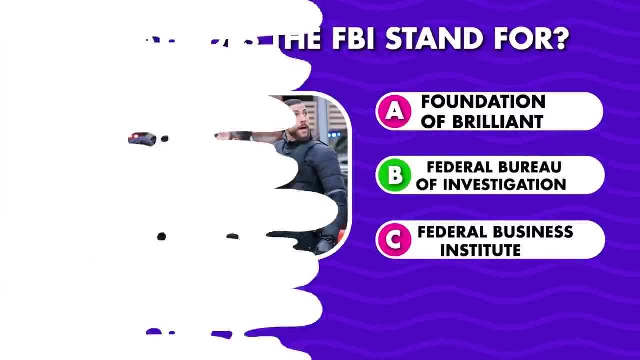 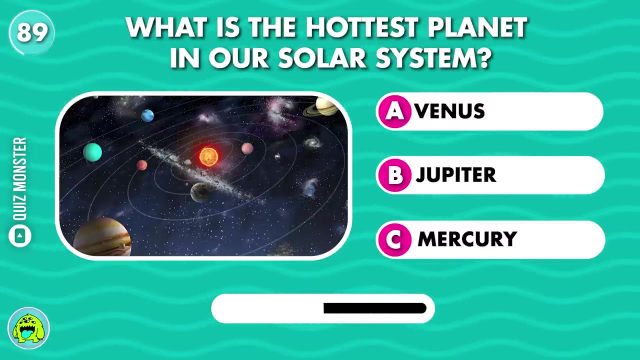 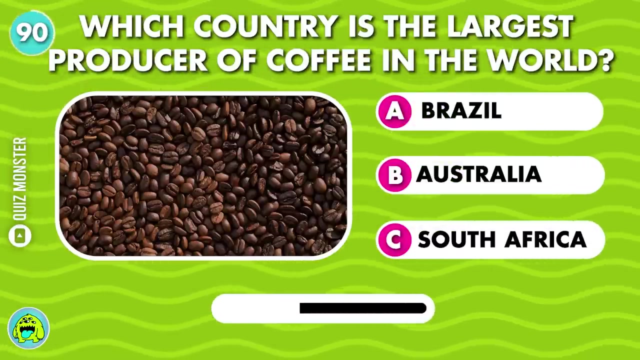 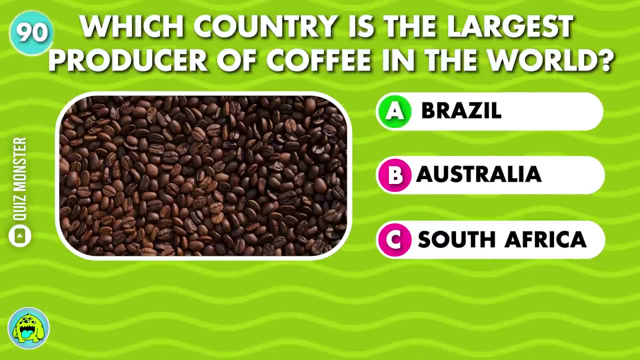 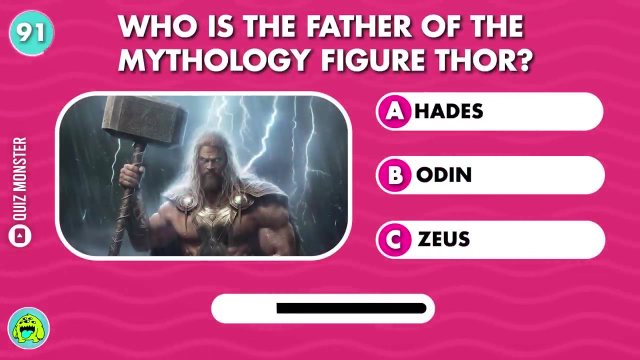 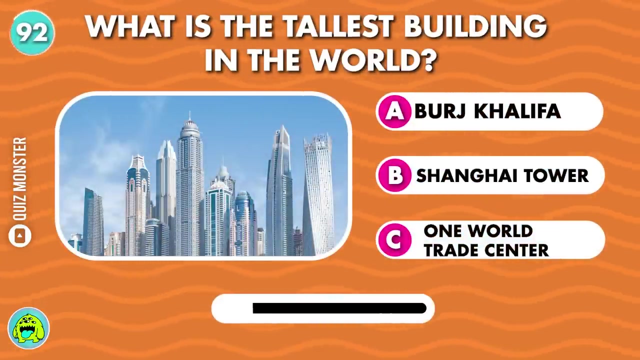 Venice, Venice, Venice. What does the FBI stand for? Federal Bureau of Investigation. What is the hottest planet in our solar system, Venus. Which country is the largest producer of coffee in the world? Brazil. Who is the father of the mythology figure, Venus, Thor Odin? What is the tallest building in the world?